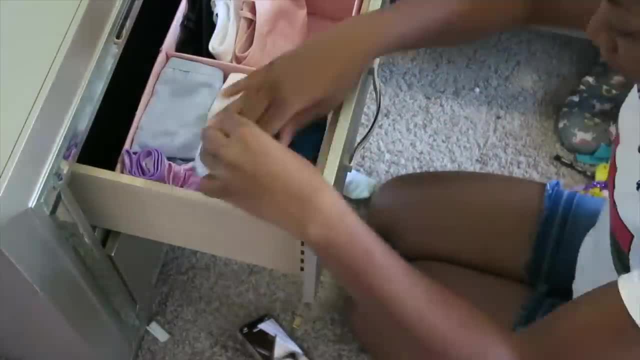 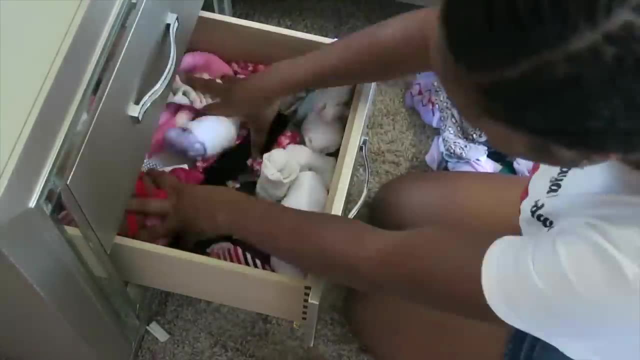 $6.99 a piece. I can't remember exactly, but they were in that range. I'm finally taking the time to go through her underwear and sock drawer. She has a million pairs of socks and about 600 pair of underwear. and she has a million pairs of socks and about 600 pair of underwear. and she has a million pairs of socks and about 600 pair of underwear. 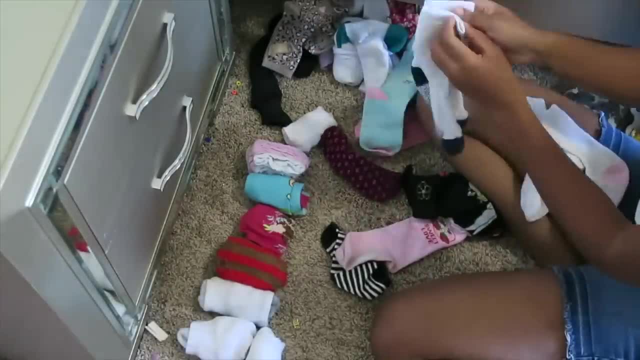 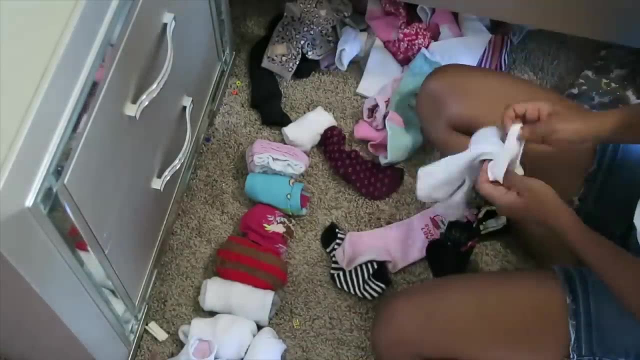 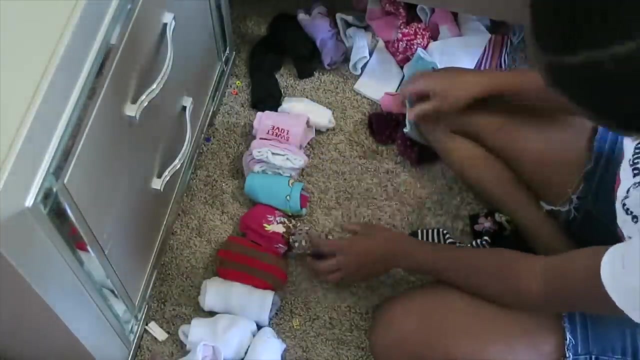 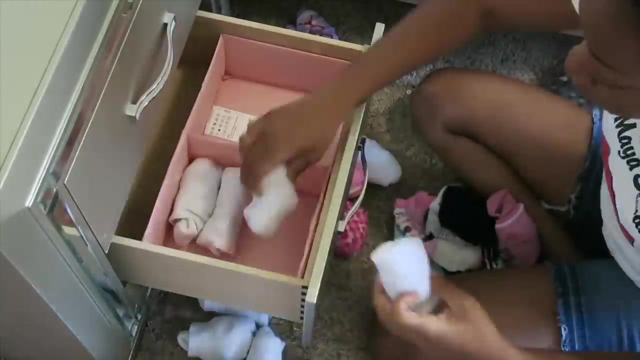 She tells me everyday they are too small. So I finally went through and picked out all the small ones, Got her some new ones, Kept the ones that fit, And we are organizing them nice and neat in the drawers. Music. I don't know why my mind thinks like this, but I felt some kind of way when I was 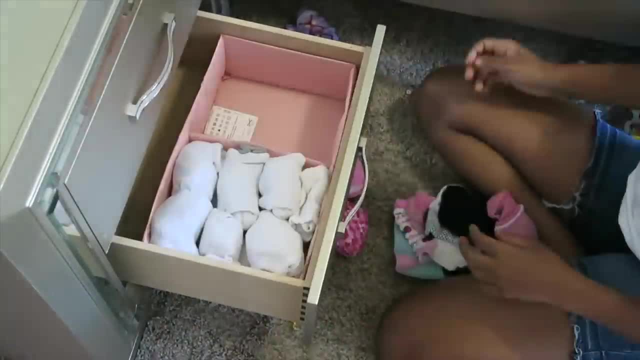 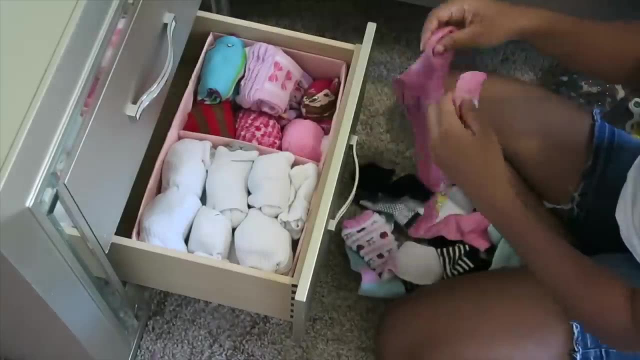 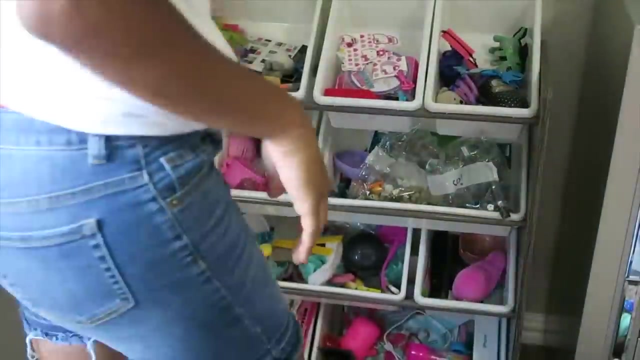 the white socks from the colored socks. I only did that because sometimes she needs to wear white socks and I figured this would be easier for her to pick them out. I promise y'all I'm not a colorist, So we're just gonna ignore the fact that my red underwear made a very large 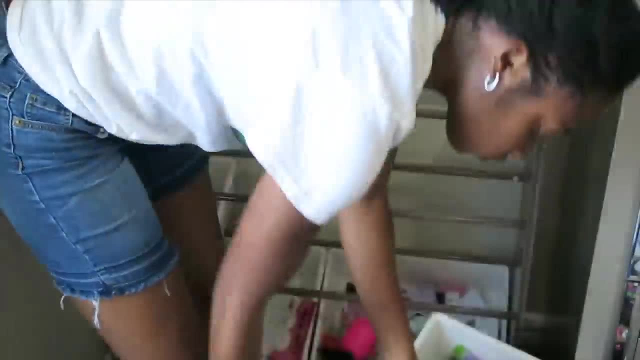 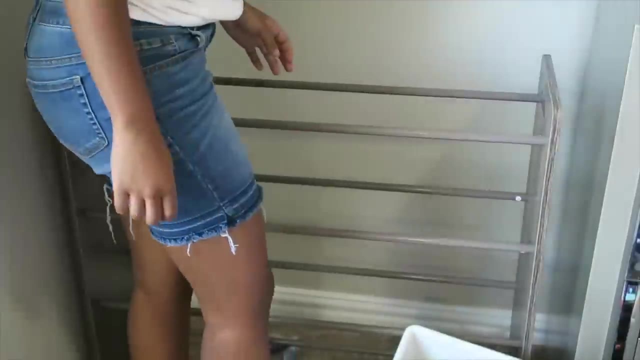 cameo in this video. We're just gonna ignore that. We're not talking about it. I do want to shout out the subscriber that suggested I just get rid of a lot of things and declutter- really declutter- her toys. I've tried that in the past and 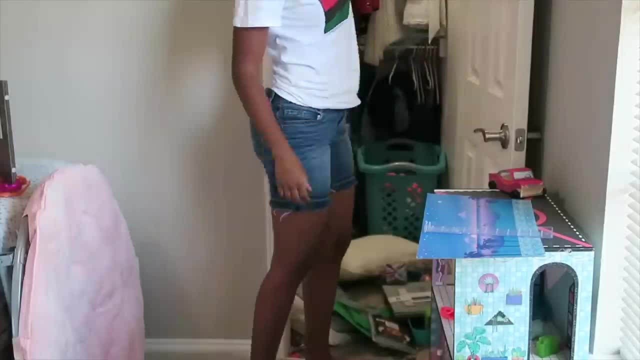 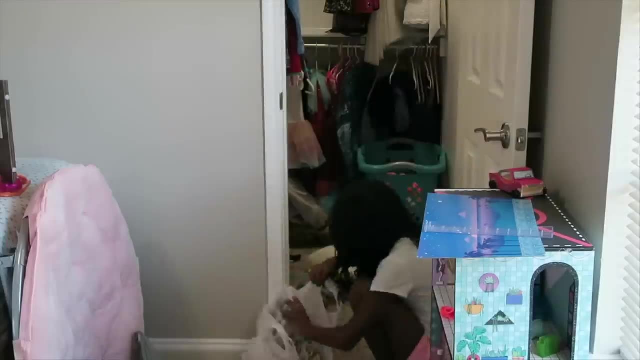 she just cries and she needs everything. but this particular subscriber really gave a suggestion on how to do it with love and that really worked for Chloe. She didn't really feel like she was throwing things away or like she was being punished. She kind of just understood. We really had a conversation. 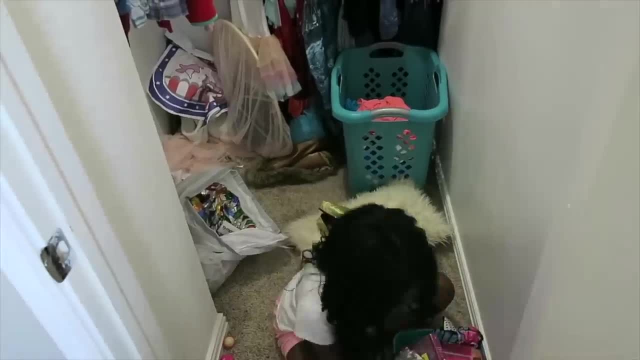 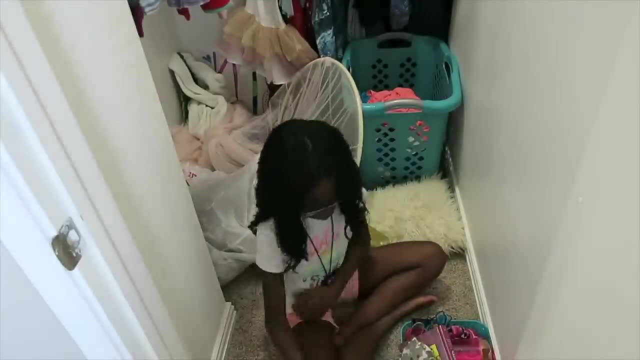 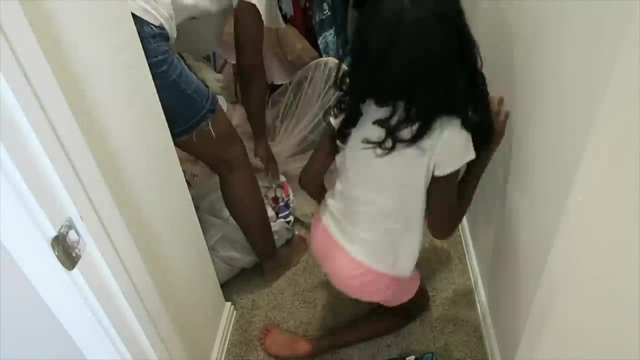 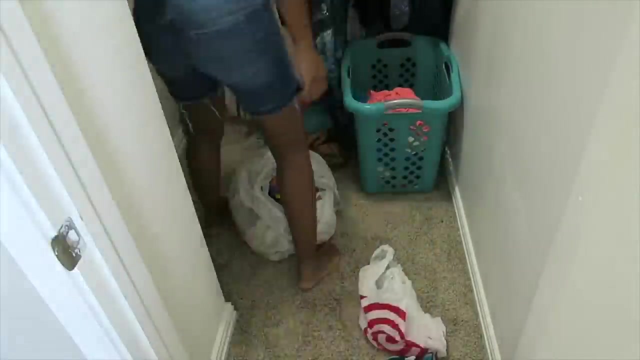 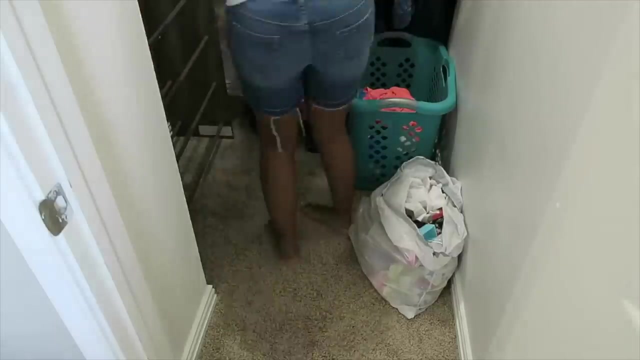 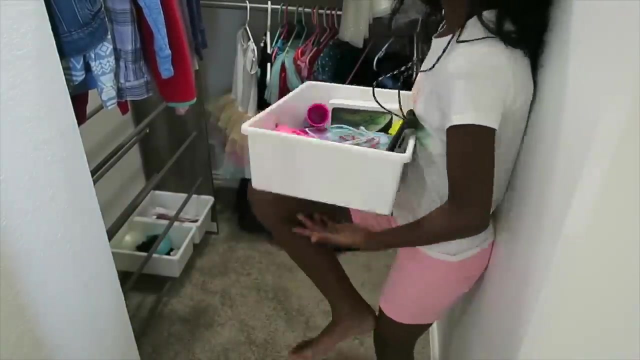 things, and that really made it easier for her. So thank you so much for that suggestion. So I decided to take the whole toy rack out of the main part of her bedroom and whatever she decided to keep was going to be nicely organized in the closet. 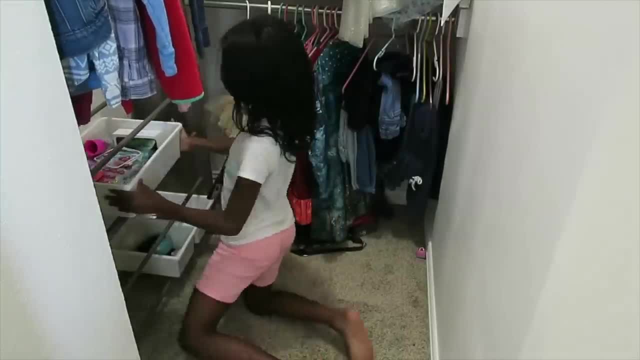 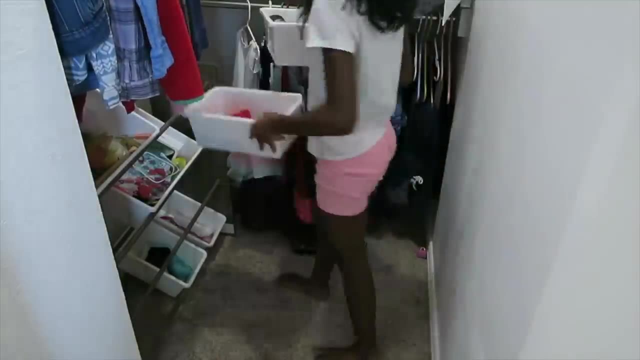 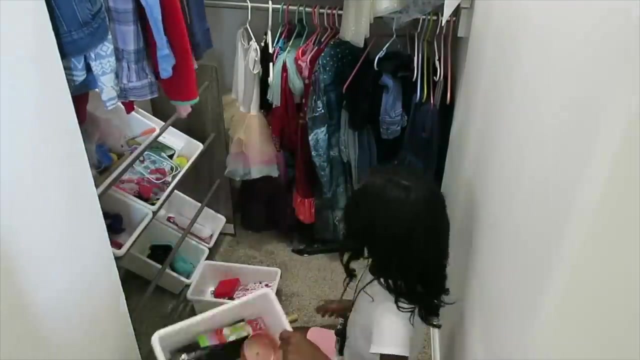 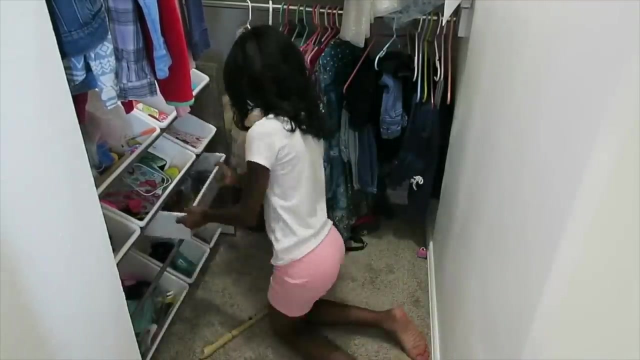 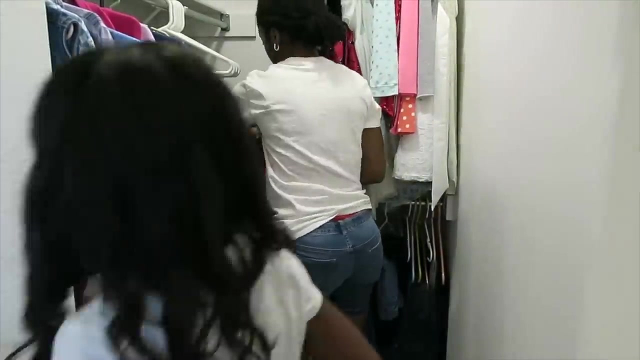 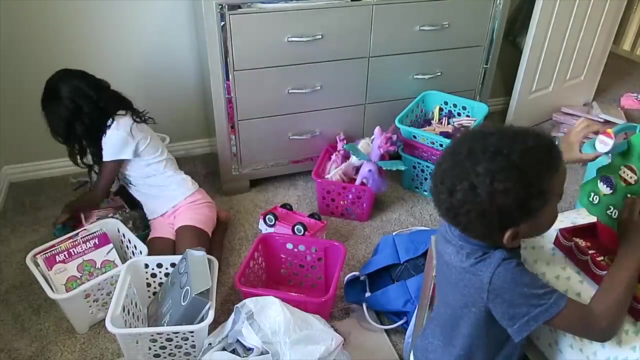 That will give her extra space in her room and I'm hoping it will be able to help her keep her toys more organized and just out of open sight. I'm really proud of my Coco Bear. She did a real good job organizing her things and she did a 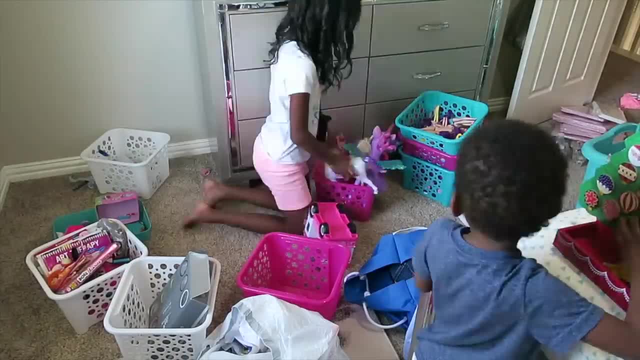 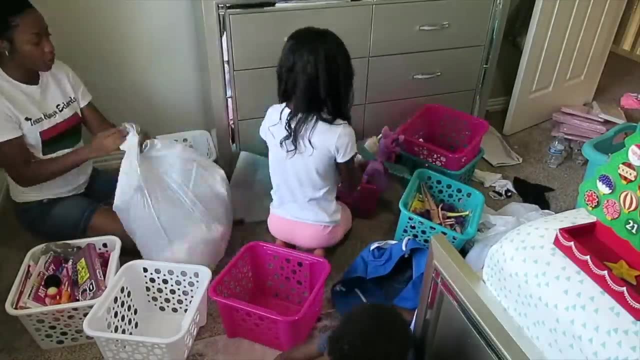 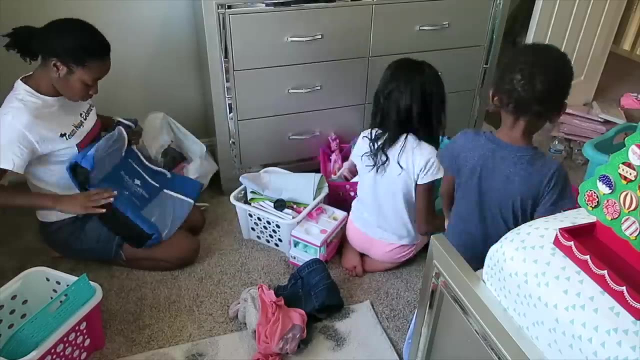 really good job, just kind of picking things and letting go of things. All those empty bins- you'll see me stack them up- and that big bag of stuff. those are all things she's gonna donate. I'm really proud of her. Mind you homeboy is over there in the corner making more mess and living his best. 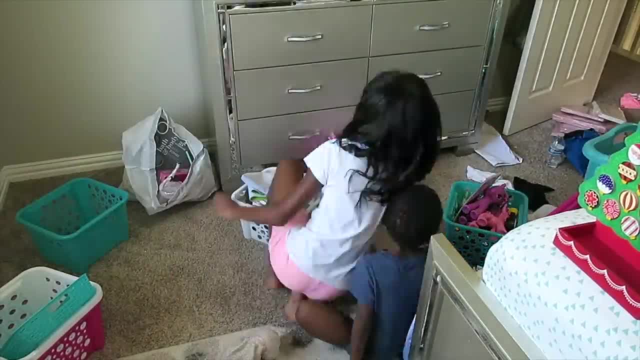 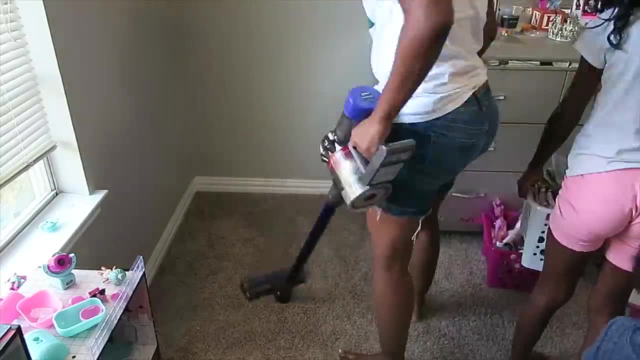 life. I really love my kids, So I wanted to do something really special for her. I wanted to do something really special for my kids for back to school, So I decided to create a little reading nook in Chloe's room. I got her a cute pink chair from Aldi with. 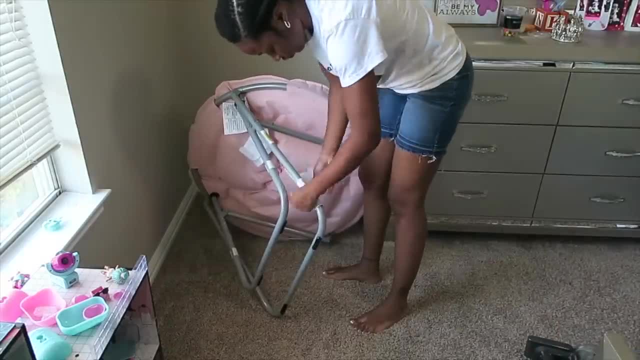 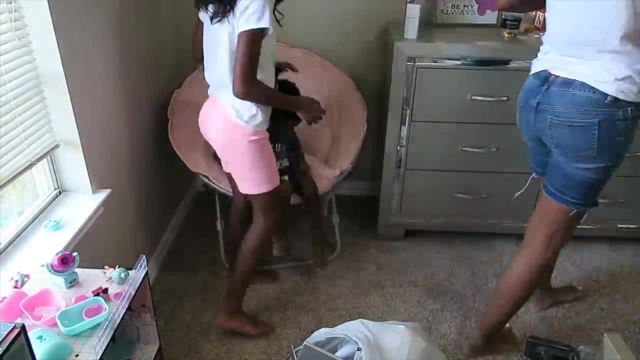 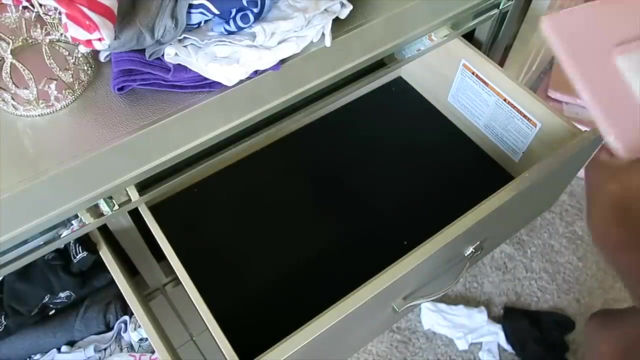 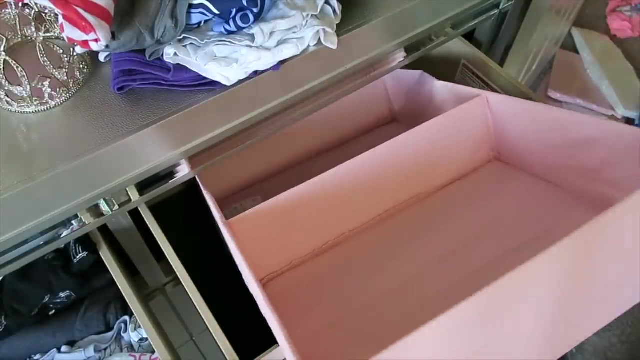 a matching lap desk and I let her pick out a portrait for her wall from Ikea and she loved it. you guys, My baby loves to read, So, disclaimer, these are the largest size drawer organized from Ikea. These ones were- I think they were- $7.99.. They're either $6.99 or $7.99. 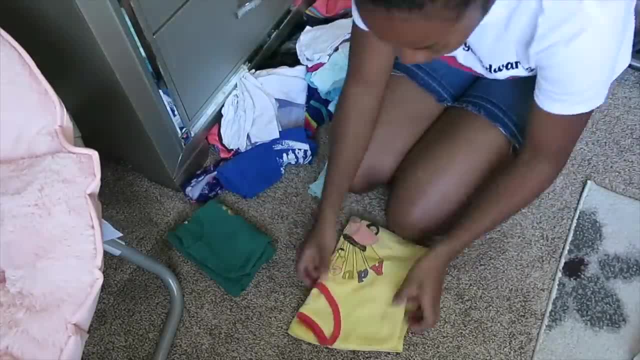 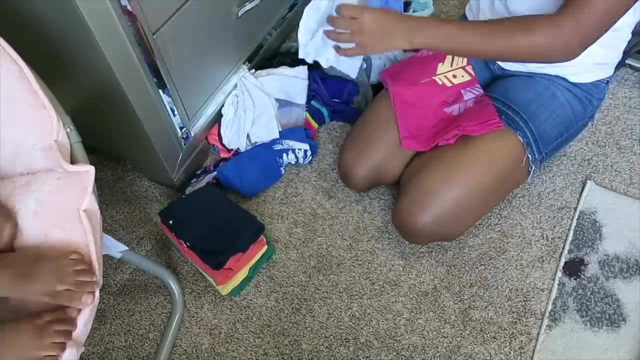 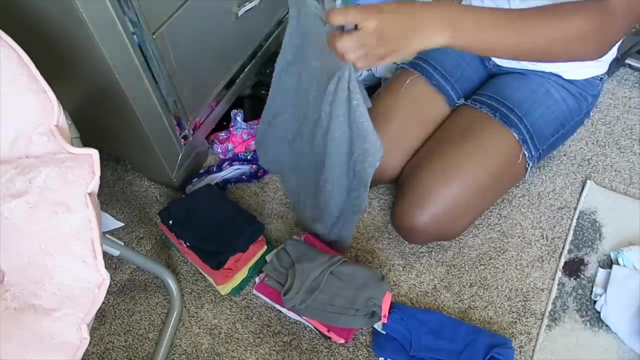 and they were like a quarter inch too small for my. rather, they were a quarter inch too big for my drawers. So make sure you have measurements of your drawers if you decide to go get them. They fit perfectly in the Ikea drawers, of course, but they were like a quarter inch too small for. 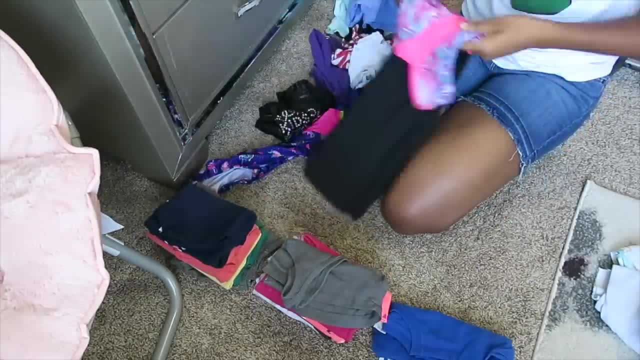 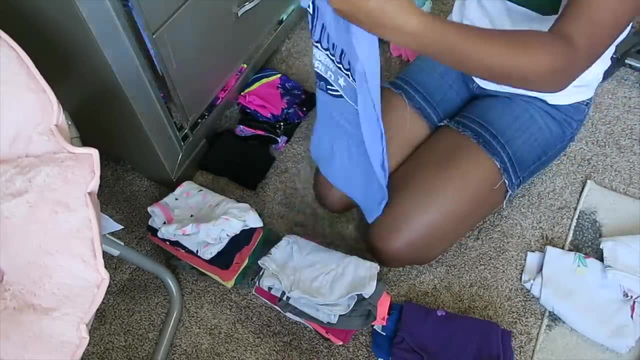 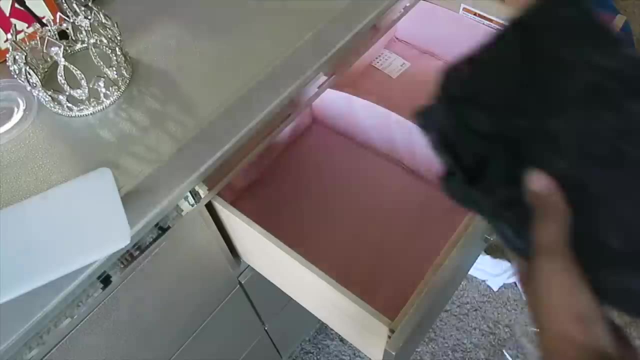 mine, and don't worry, I made them work, but I'm just putting that disclaimer out there. So again, I'm just decluttering all her drawers and reorganizing the clothes. I'm getting rid of all the t-shirts that are too small and putting all her new t-shirts in the drawers, Just to let. 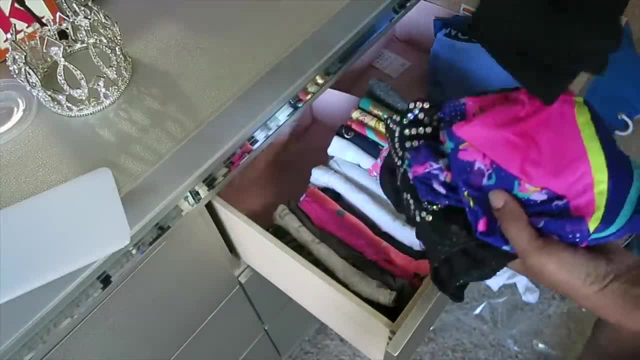 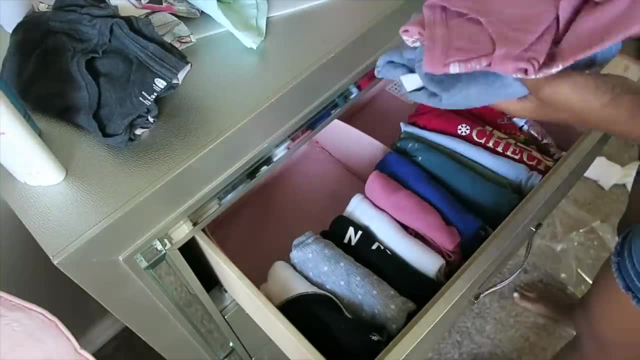 you guys know, I did go to Old Navy's. They were having a major sale: $4 t-shirts- okay, $4 t-shirts, and Chloe wears a size 10-12.. So if you need to get some clothes for your kids, head to Old Navy. 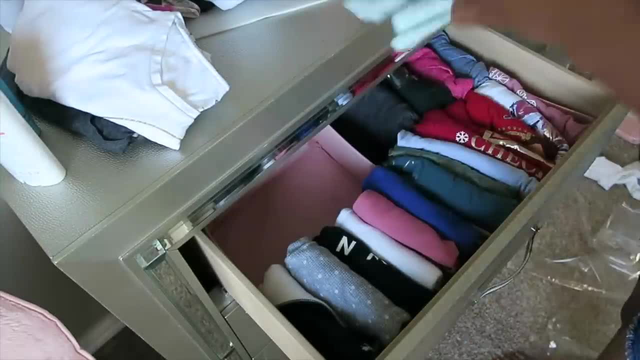 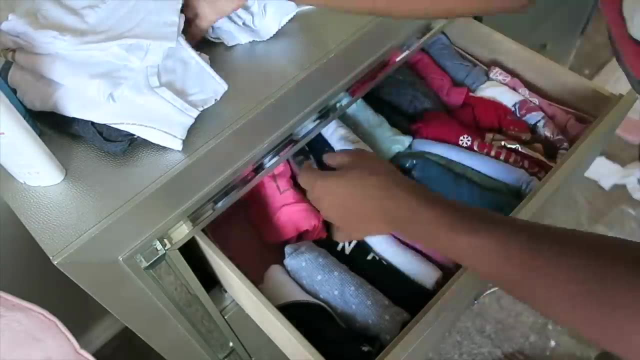 This drawer right here has all her long sleeve shirts. I didn't really declutter and get rid of anything in that drawer yet because we just haven't gotten to long sleeve season yet, but I will go back over that drawer. Most of those shirts are size 10-12, which is what she's wearing now, so should. 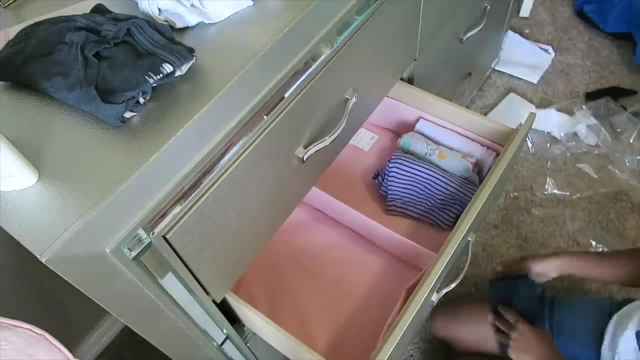 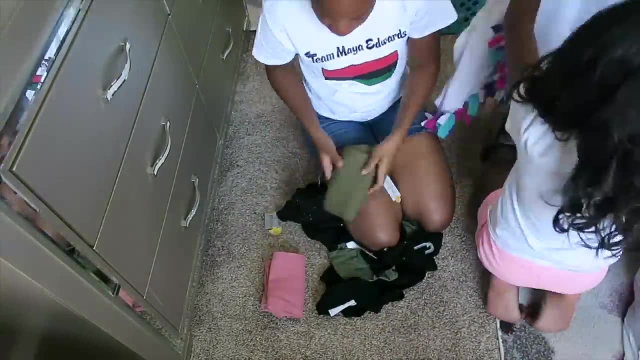 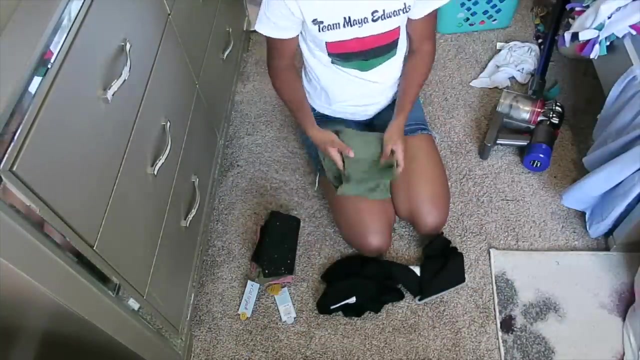 still be able to fit most of them. I also wanted to mention that Old Navy have $4 leggings as well, so if your little girl likes wearing leggings, they're $4 at Old Navy's. I also like the Kat & Jack brand leggings from Target, and I think theirs was $6, so not a bad. 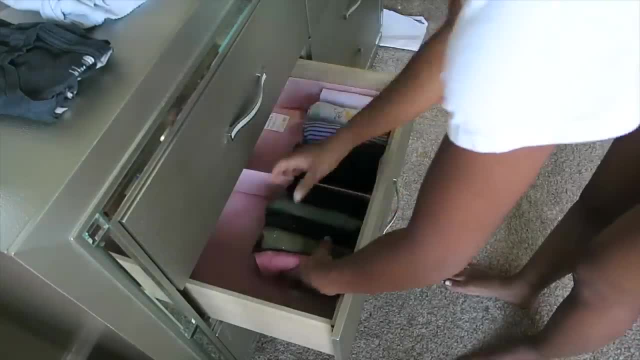 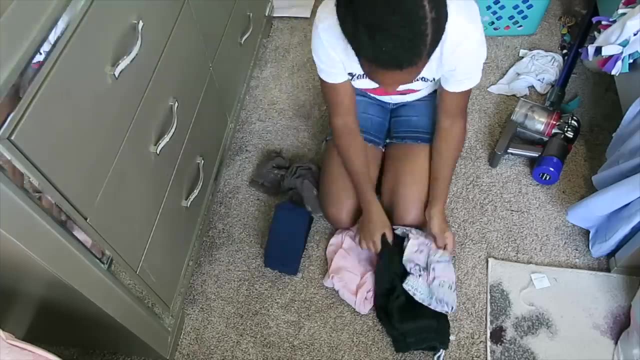 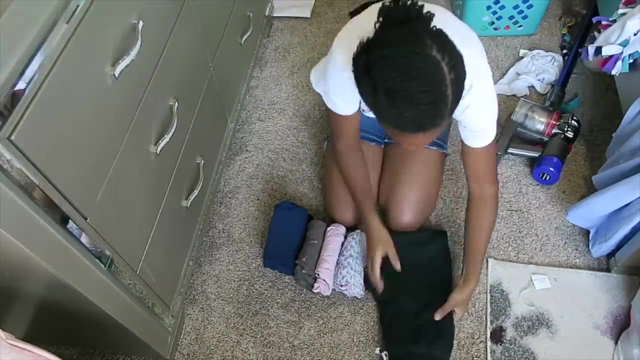 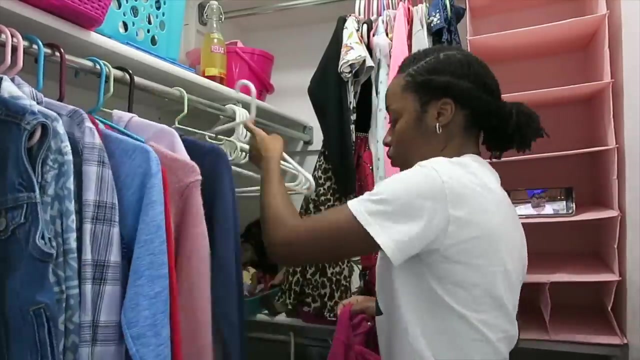 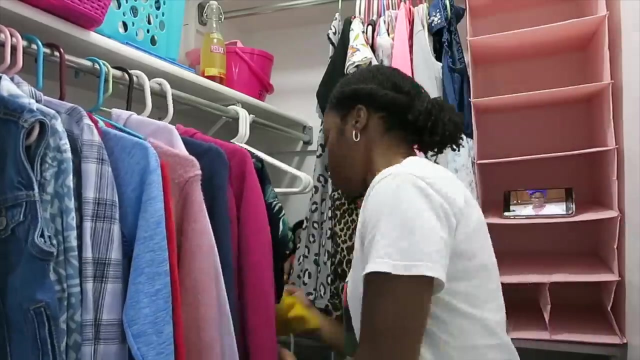 price She's set with her leggings. So shout out to Chloe, because she did a great job cleaning out her closet. The floor is nice and clean- You'll see that in a second- So now I have plenty of space to just organize her clothes Right now. 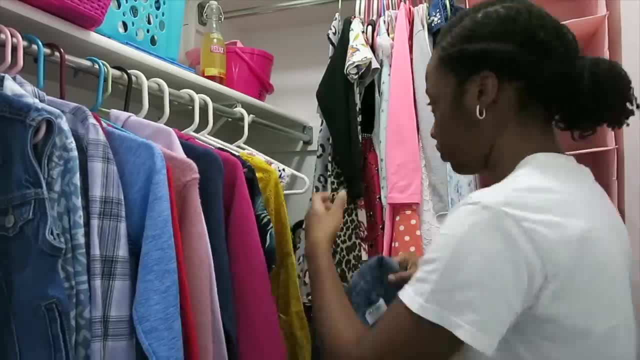 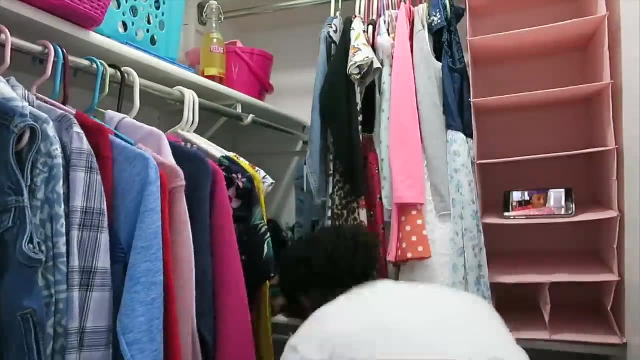 I'm just hanging up all her new shirts. I'm actually hanger hunting right now trying to find all the loose hangers so I can hang up her new clothes. You guys, I got that cute little jean dress from Old Navy's. It was on sale for $20 and you know original price was like $32.99 or $34. 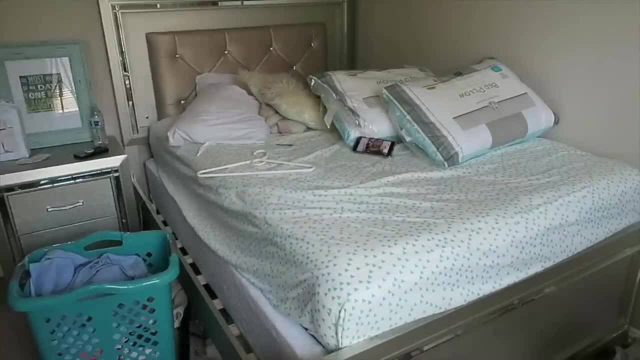 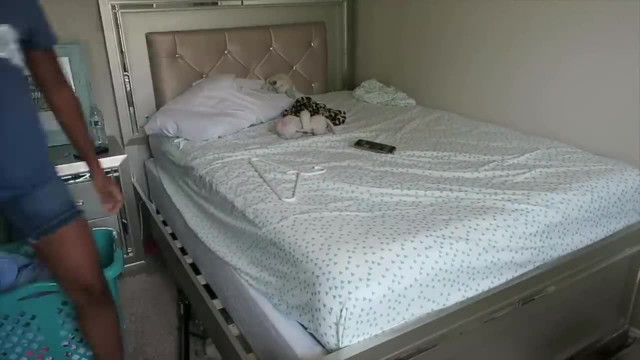 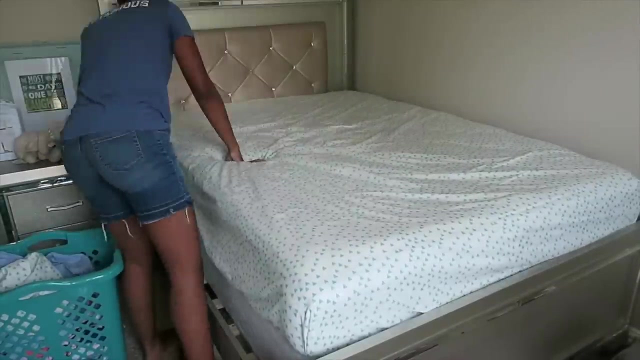 something. So check out Old Navy's. They have the good sales going on right now. Can somebody please tell me why I keep saying Old Navy with an S at the end, like Old Navy's, Old Navy's. What is wrong with me? 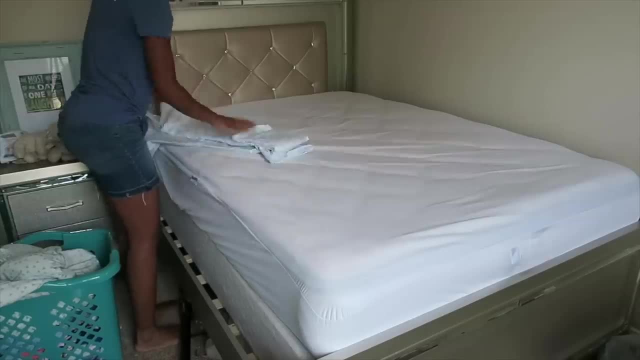 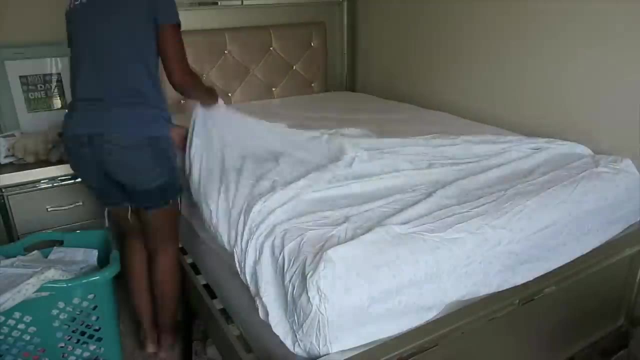 So I did get both my kids a new pair of sheets for their beds as well. I get most of their sheets, Well, they only have two. so this is their third set. I got two of their sets. from all these they are $7.99 for the full. 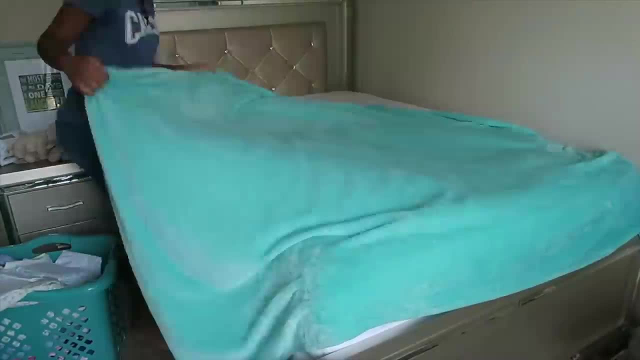 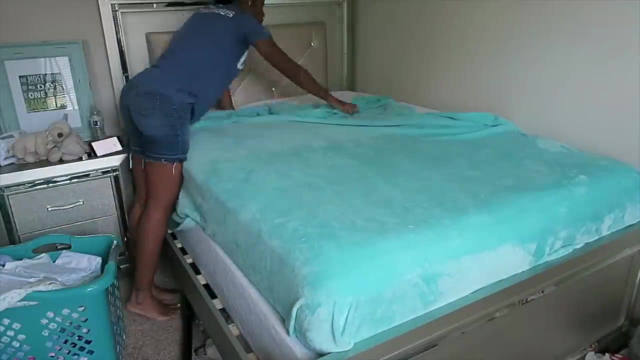 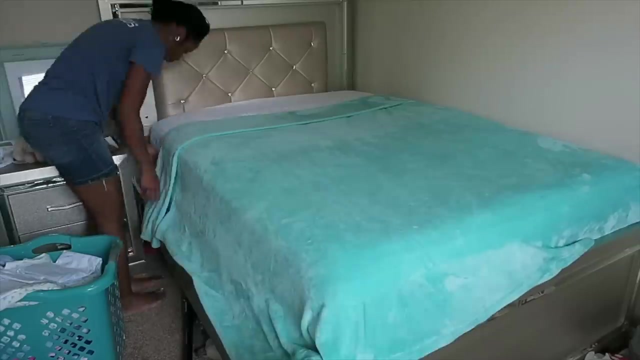 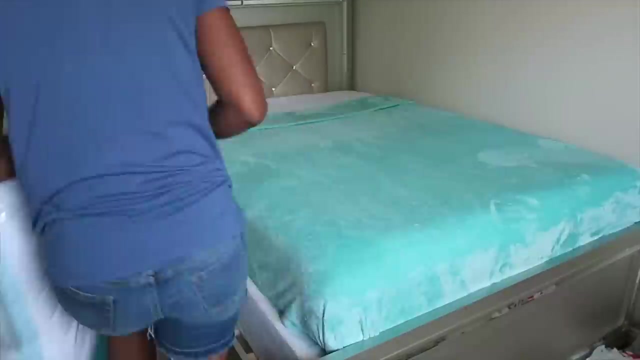 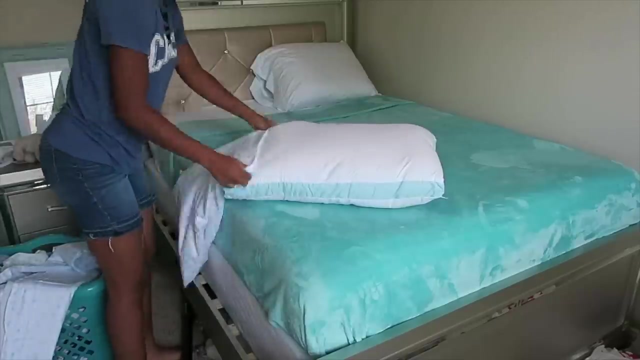 size. complete set comes with the fitted sheet, the flat sheet and two pillow cases for $7.99. you really cannot beat that price at all these- and they have one set from Target, of course. I'm burning all my good energy making this girl's bed and in about five. 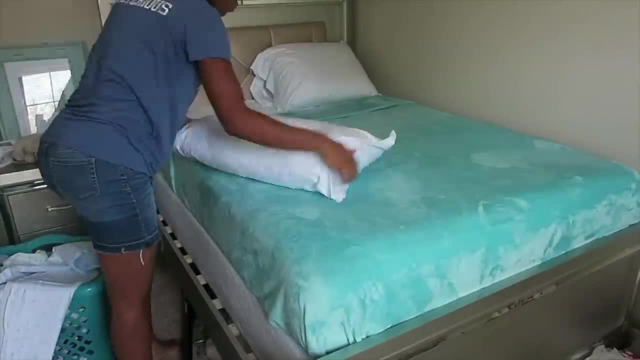 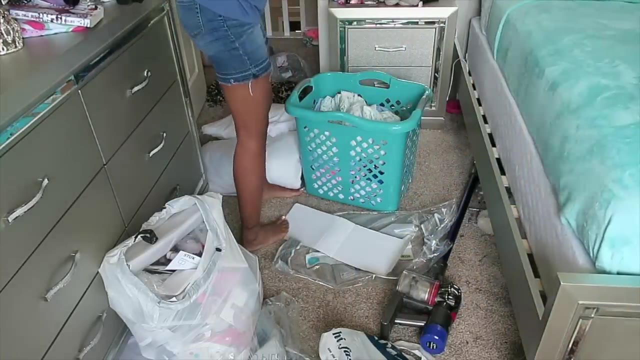 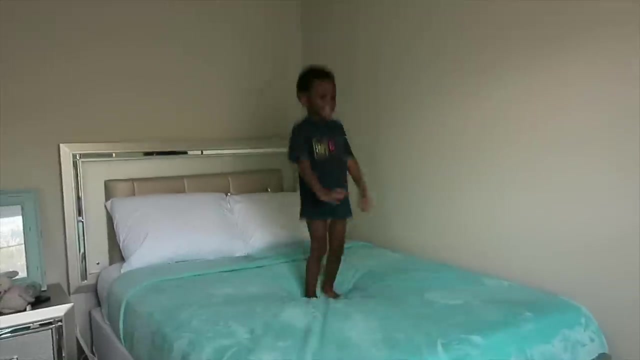 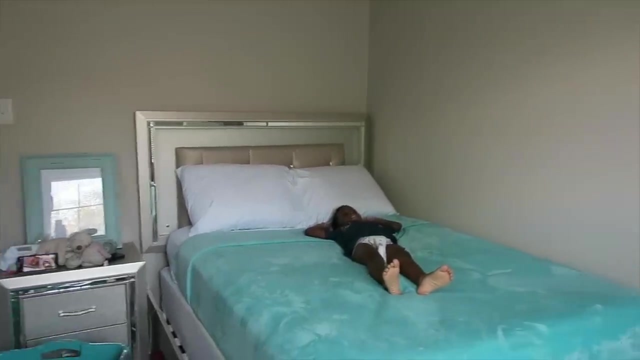 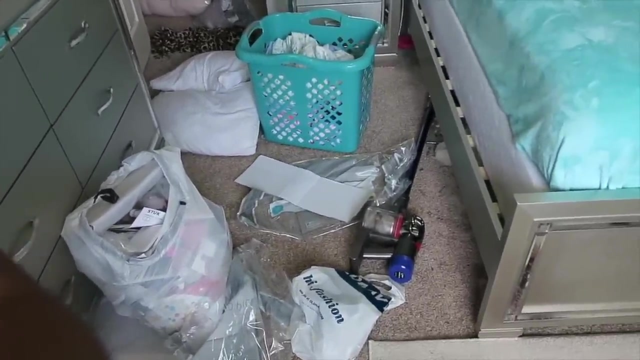 seconds. you're going to see, it was for absolutely no reason. I love my kids. y'all just made that bed. I just made this bed. oh my gosh, oh my goodness, you crazy baby. so I am just adding the finishing touches. I am proud of this girl, her. 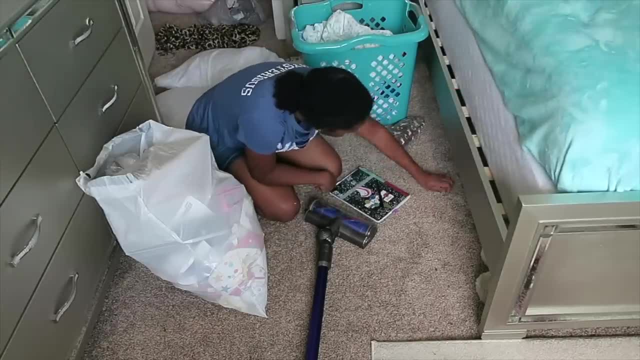 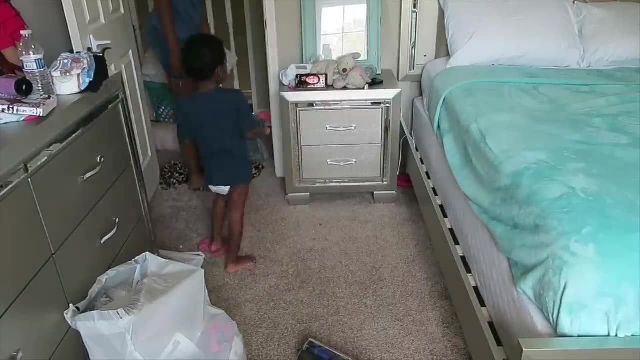 under her bed wasn't a wreck. of course she had a few little things under there, but it wasn't a wreck, and if you're wondering where she's at at this point of the video, she went downstairs to straighten up whatever toys that she was gonna keep down in the playroom. 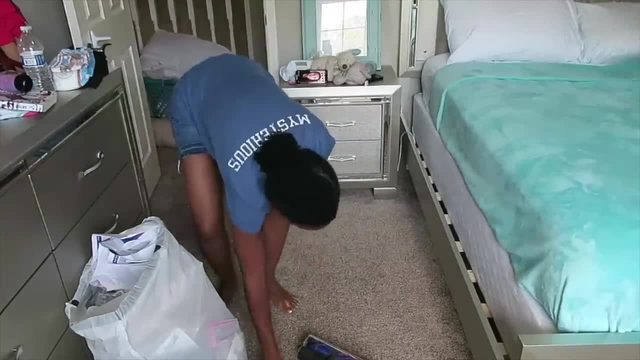 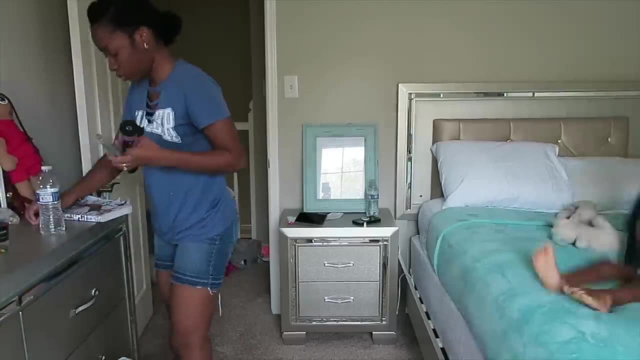 in the playroom. I told her do not go place them toys on the floor in the playroom and say they're in there, put them up, because if I go down there and they're on the floor they're going in the trash. so go put it in the playroom. 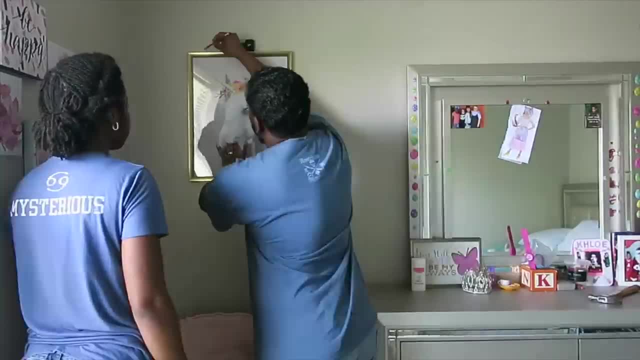 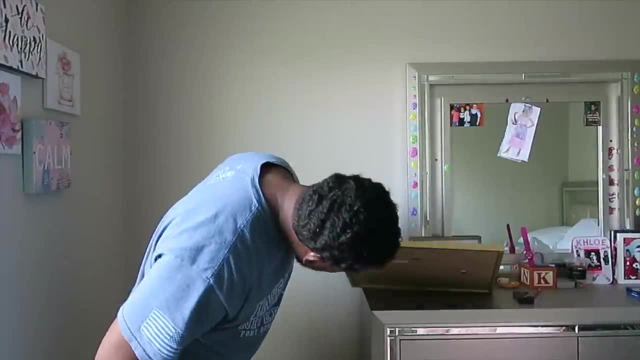 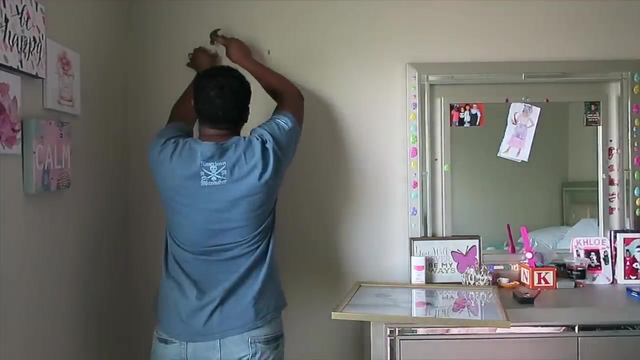 and put whatever you're keeping up. this is the picture that Chloe picked out from Ikea. it's really cute. they have these cute posters in Ikea. most of them range. they were around $10, this one was $10 and the frame was $12. it's a unicorn picture which is like perfect for. 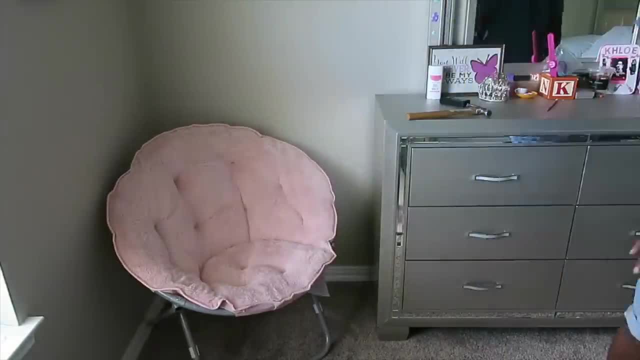 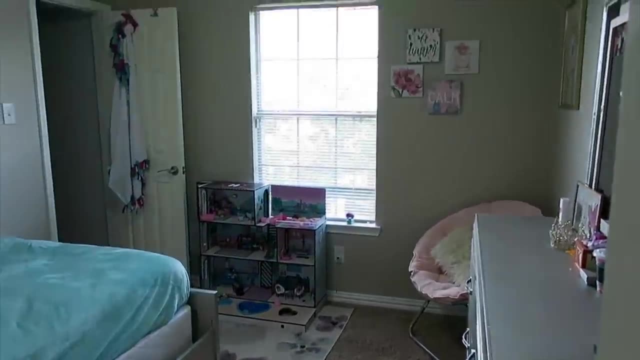 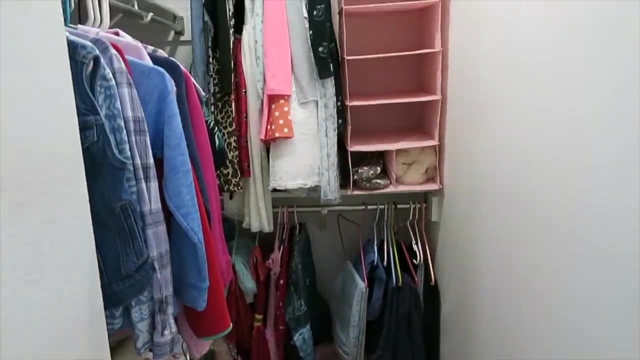 her. it suits her personality so well. so here's the room reveal. I'm also proud to say that she's been doing a really good job keeping it up. good job, Coco. mommy loves you. but I also had to say thank you so much for all of the subscribers at this point when this 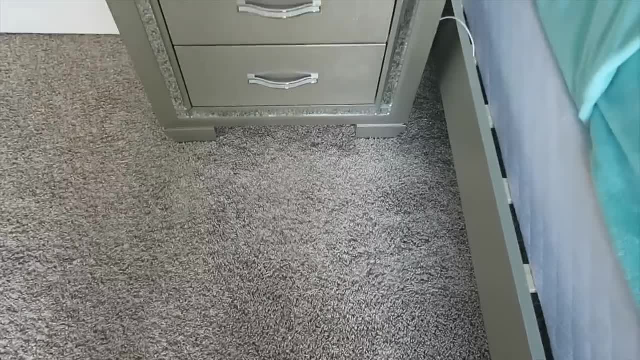 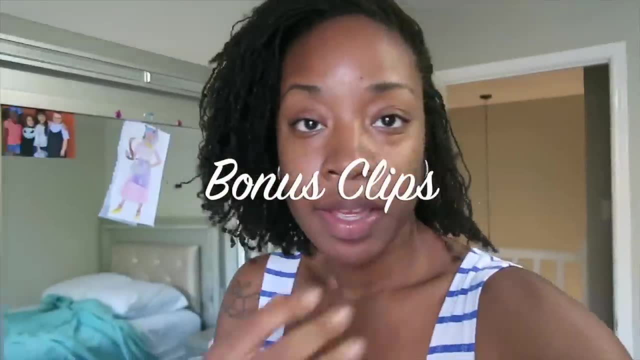 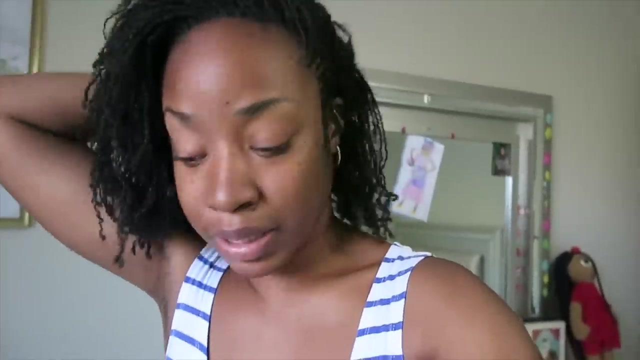 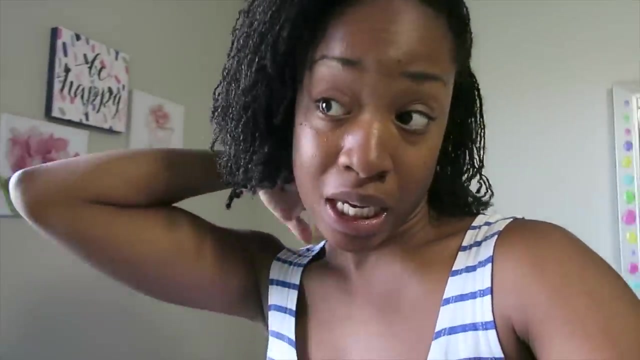 video was filmed. we were on our way to 5am, but we have hit that. so thank you so much, guys. I really appreciate you all. right, guys? so you guys saw the video in the room reveal. I am: look, this is real life for ya. Y'all love the realness of the video, so we are picking the clothes. 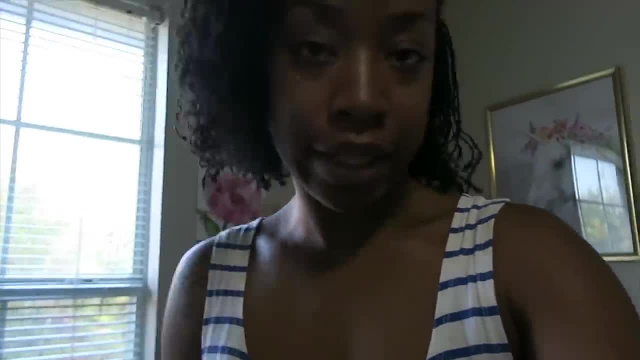 before we take that out, let me not ask you to put nothing in there. yet we're gonna pick out the outfits. I'm going to approve the, as we have jumpers- wanted to show you. You have to brighten up your workup and you know we do need to take out too many tactics on this video, so anyway, alright. so today I'm going to air it off. now Shake some air l candle and dress all your hair pur opinions- unwind ski. 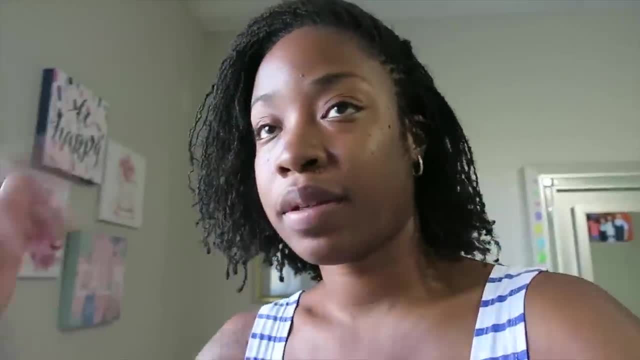 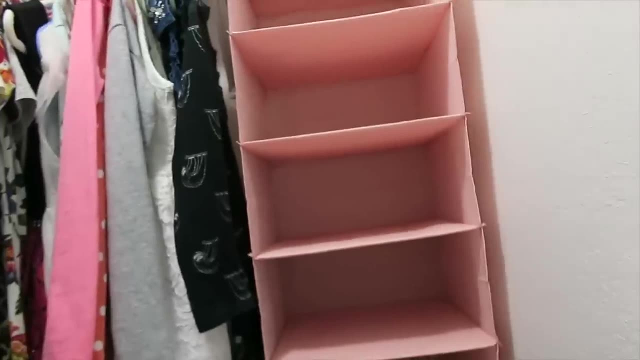 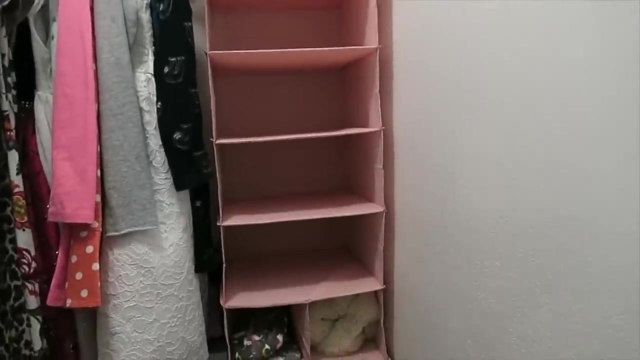 the outfits, then we're gonna pack the clothing cubicles. so i'm gonna show you guys what we're doing. right now. i'm out of breath and i was literally just laying in the bed so i don't know, but i got one of these um clothing cubicle things for each of my kids, so that so getting them dressed. 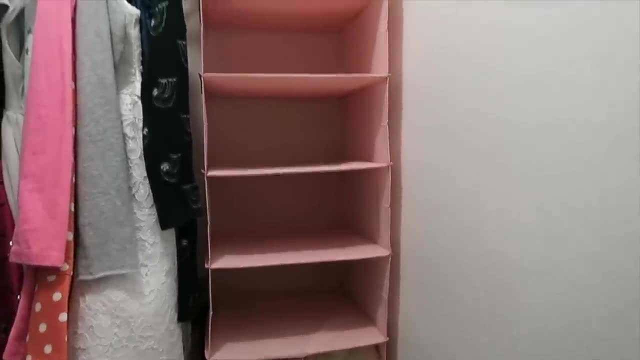 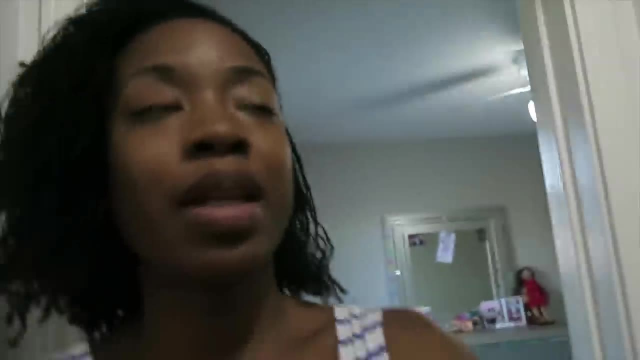 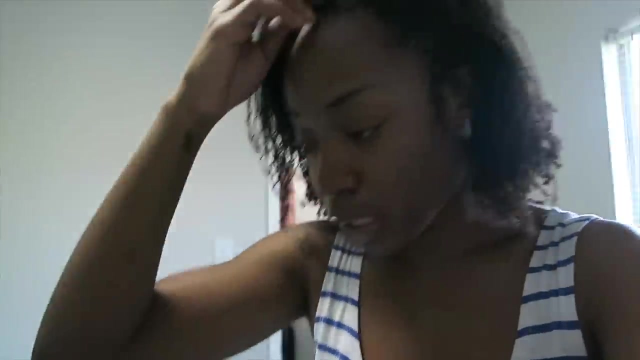 for school will be easy. i'm gonna show you what we pick for chloe y'all. i'm out of breath like a real fat kid- oh, that was mean, i didn't mean it like that, but just like a real out of breath person, um. so of course, chloe's nine, so she's gonna pick out her outfits and i'm gonna 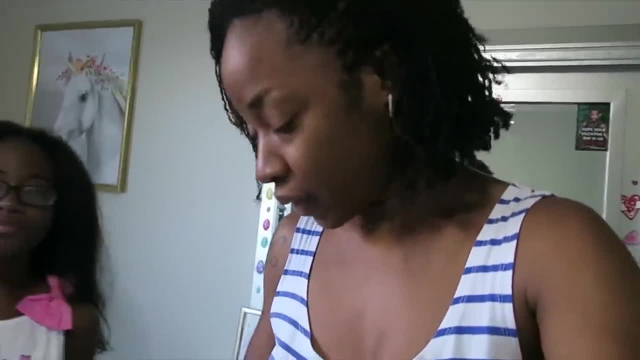 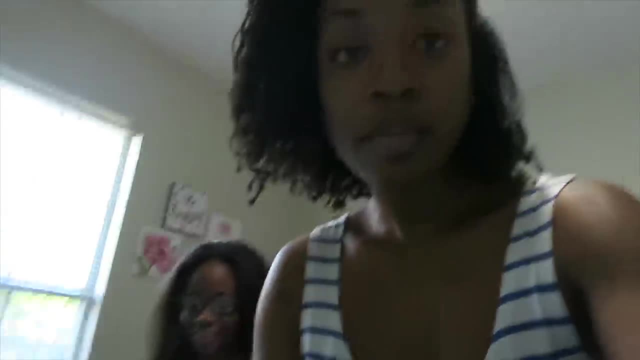 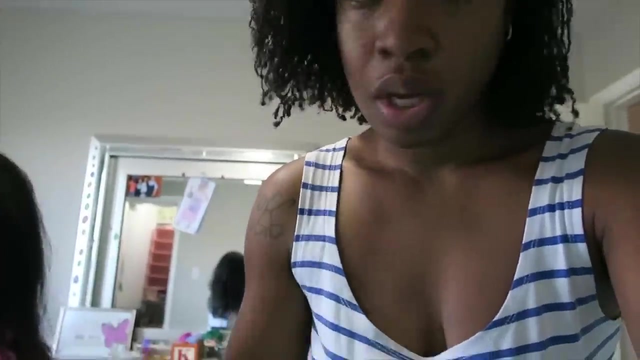 make sure that i like them. so what's the first outfit? hi, oh, chloe says hi, i'll get that hair together in a second. so the first outfit is gonna be: her and her brother are gonna be matching tomorrow because they have the same t-shirt. i got it from oh navy. oh navy got a big sale. oh yeah, open up your first. 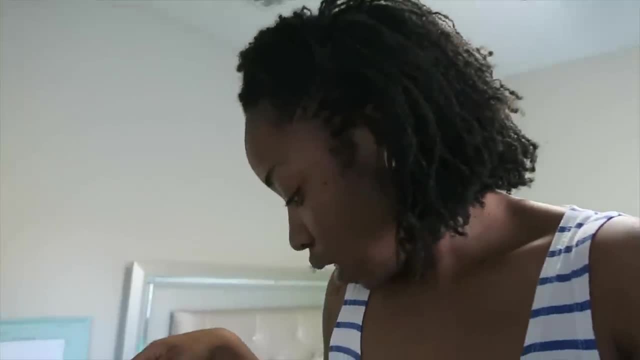 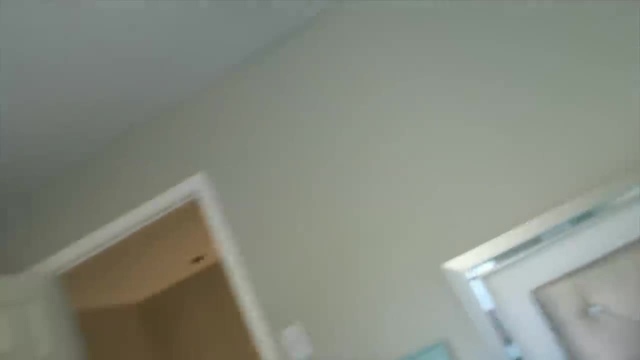 outfit and we're gonna pick some outfits. let's pick some outfits and we'll go from there. it's gonna be 100 degrees every day. pick out all her clothes. so her and kingston will both be wearing this t-shirt. they both have the same t-shirt. 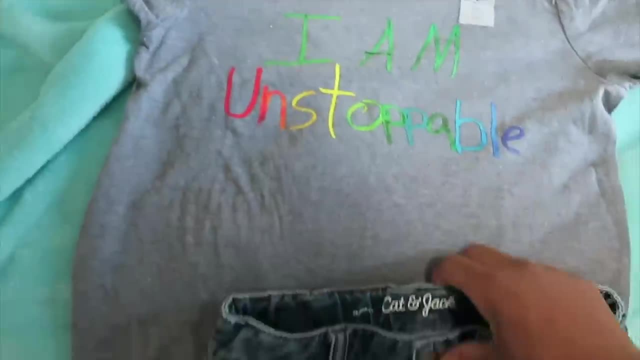 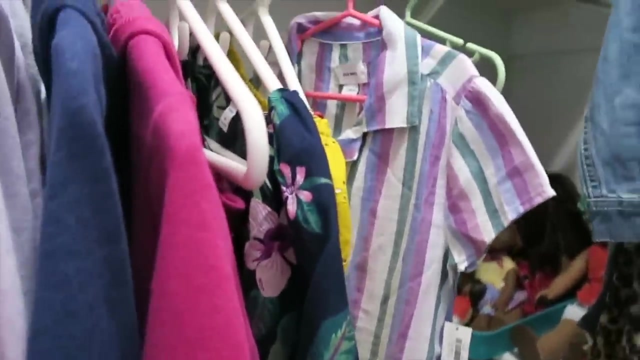 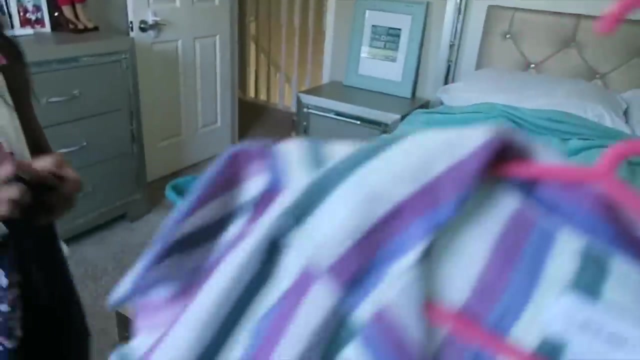 that's why i'm out of breath, says i am unstoppable. i thought it was so cute, so of course i got it for both of them, and she's gonna be wearing that with a pair of shorts. what else, girl? all right, so we got this, okay, so you could put that shirt out. that's two, three. 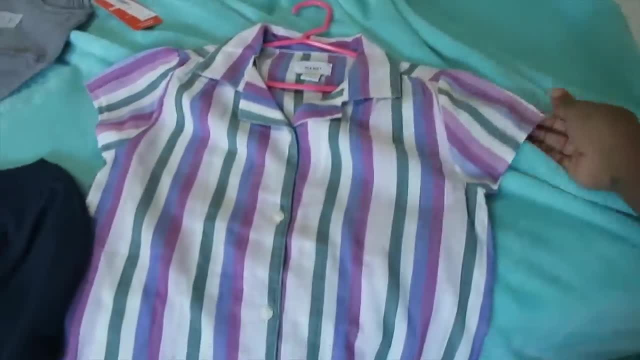 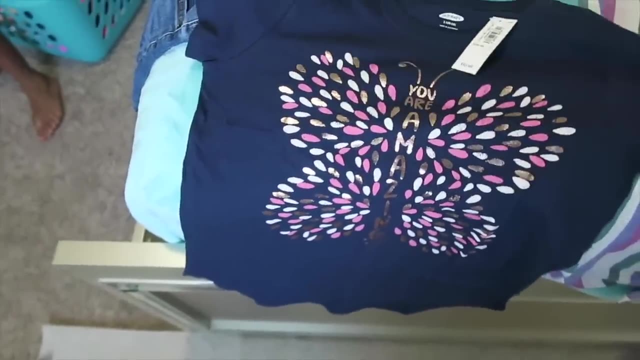 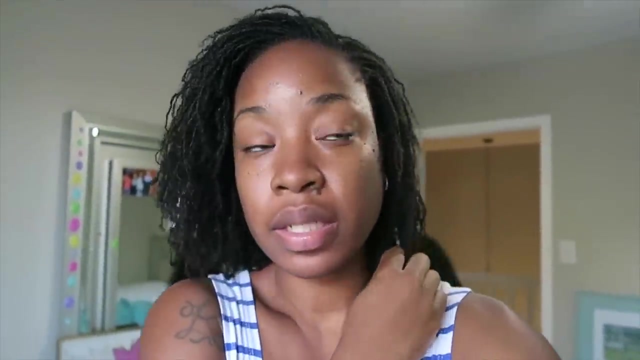 so we got this cute little shirt. it's a button up with a little tie in front, and this one is also from old navy that says you are amazing. so shout out to yesenia from yesenia, yesenia's. it's a mom's life for this whole little organization. 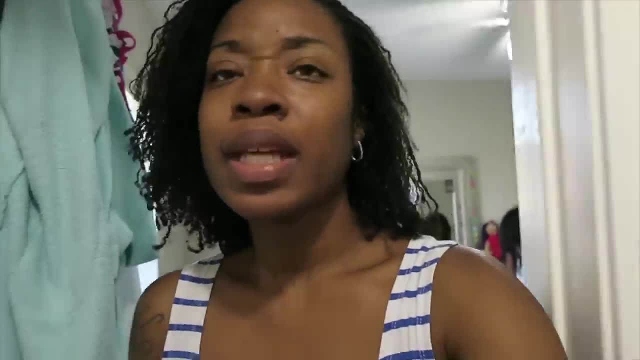 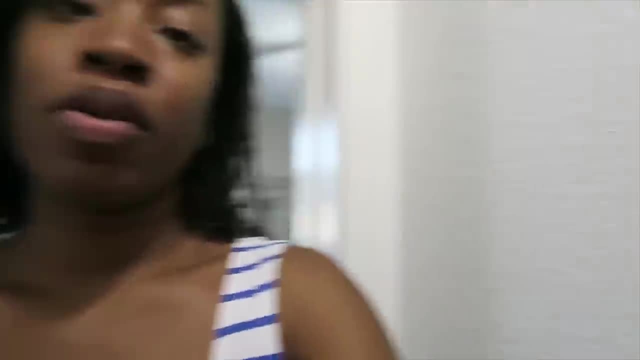 idea for getting the kids ready for school. um, that's not the first time i saw it, but i just watched her back like getting the kids ready for back to school video and i saw her organizing her daughter's clothes in one of these and i said i have to get her ready for school. 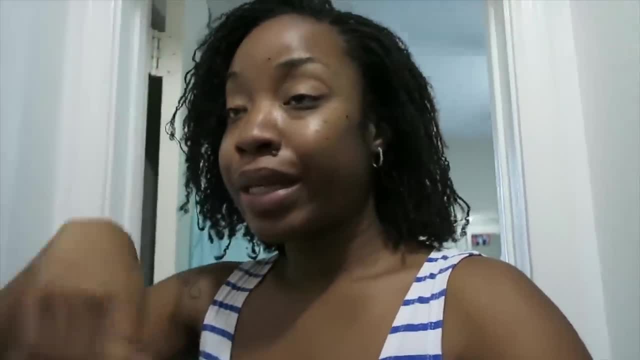 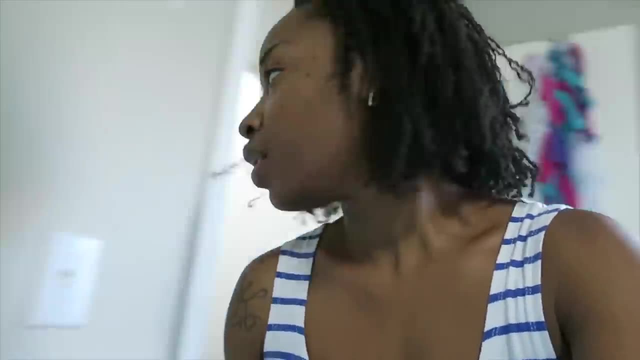 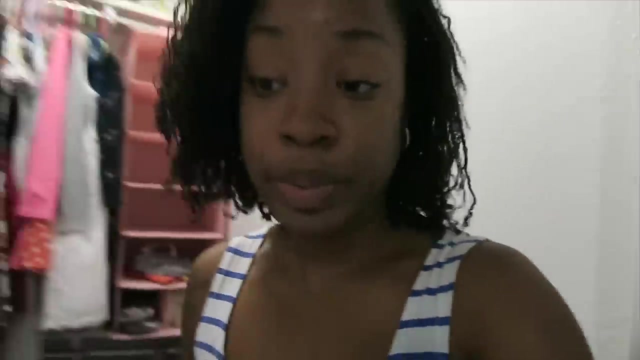 i have to go get one that will make our lives so much easier to get this girl's clothes together beforehand, because last school year that was a situation between her picking her clothes and her dad picking her clothes, y'all. sometimes she was going to school with pajamas. 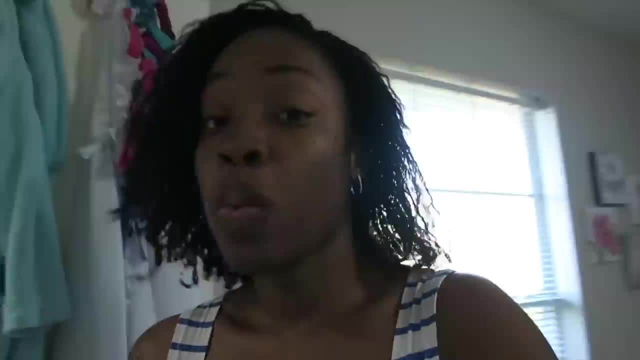 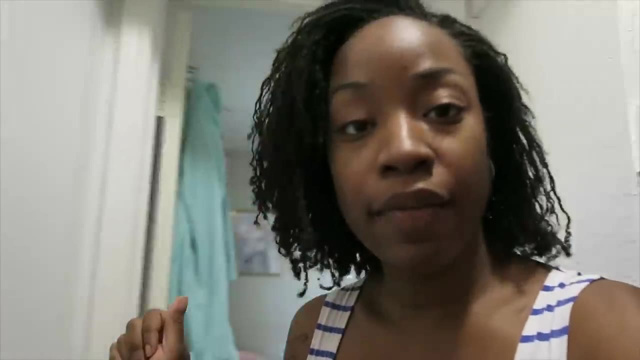 on um, because i'm not sure why the two of them don't know the difference between her pajamas and her clothes. but now this will have it all together. so if it's one of my work days during the week and i'm not there to help her pick her clothes, 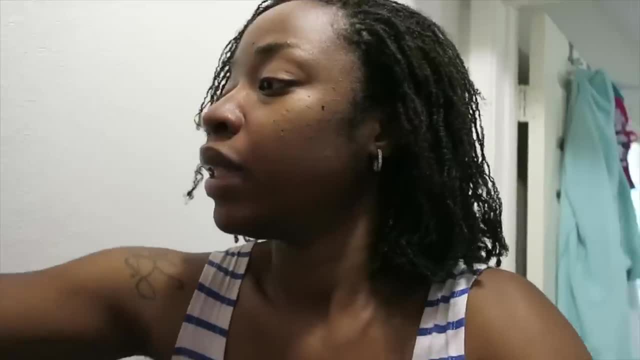 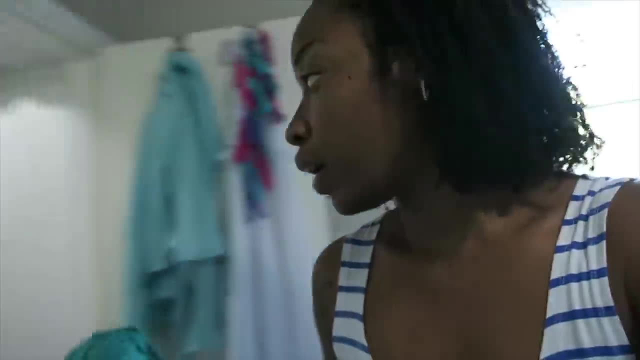 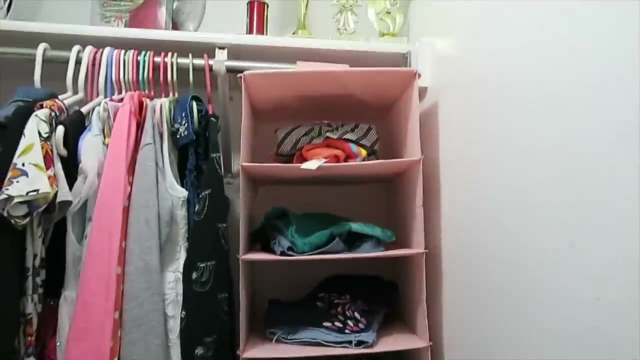 we ain't even got to worry about it. she all situated, situation has been situated and she is straight. so thank you, yesenia girl, for including that in your video, because that was very helpful. so here are all her clothes and the organizers for the week. so she's just. 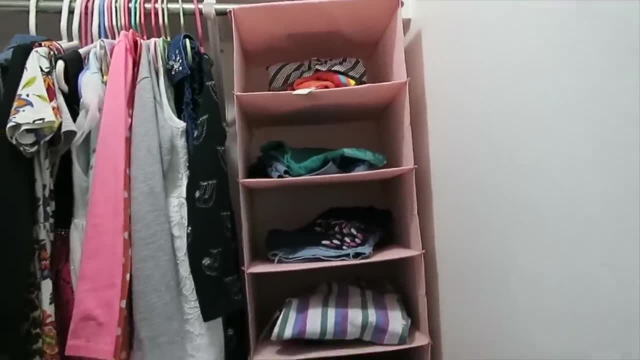 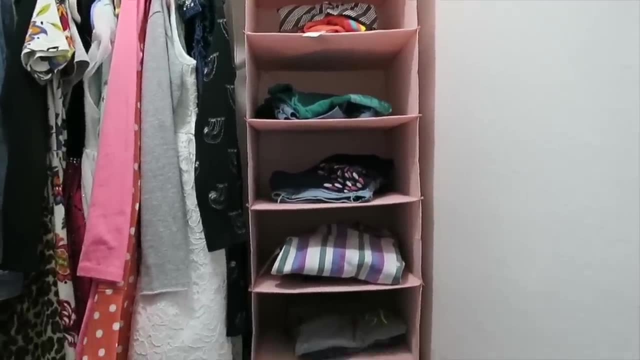 gonna pick one and get dressed. i really don't care. we don't do it in order of monday through friday: pick an outfit and get dressed. if it's in here, that means it's mommy approved and she just keeps her slippers in the two bottom sections down here. 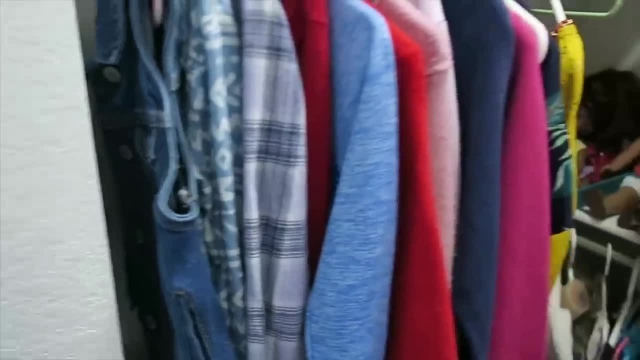 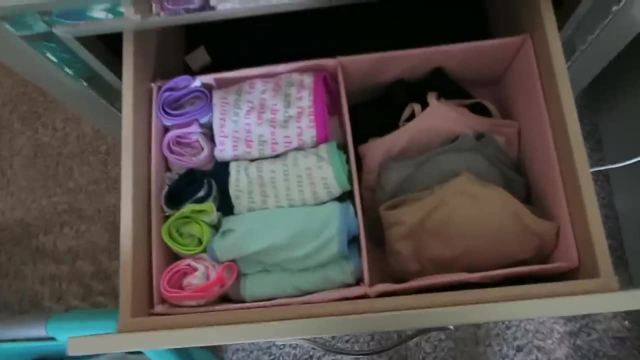 and that's it. that's it, that's all. so this is her closet. i showed you guys after shots of the room already, but everything is pretty organized, so i am loving these little organizers from ikea. they are so cute. the small ones were like 3.99. i probably said all of this in a video, but i'm sure it's one of the best i've had in the last few weeks, so i'm going to check out those. 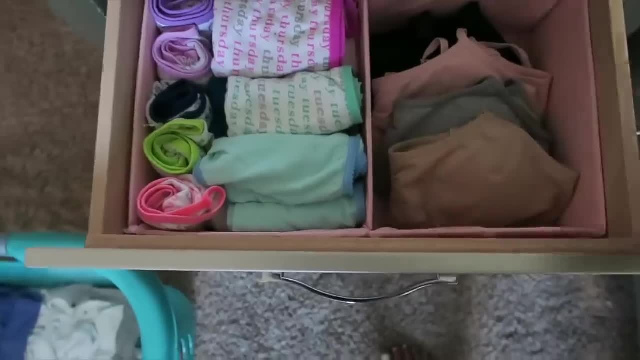 all these clothes were like $3.99. i probably said all of this in a video, but i'm going to check out those because i have a lot of things to do this year. $3.99- I probably said all this in the video, so I ain't gonna repeat myself. but